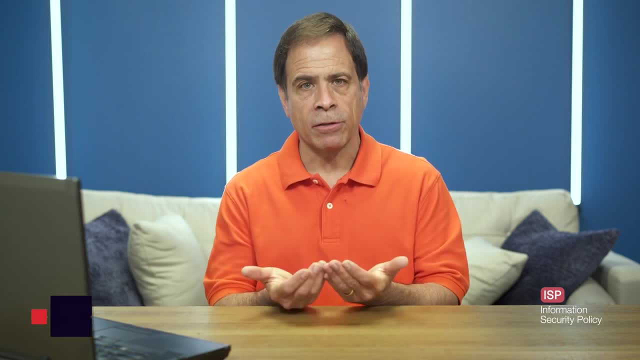 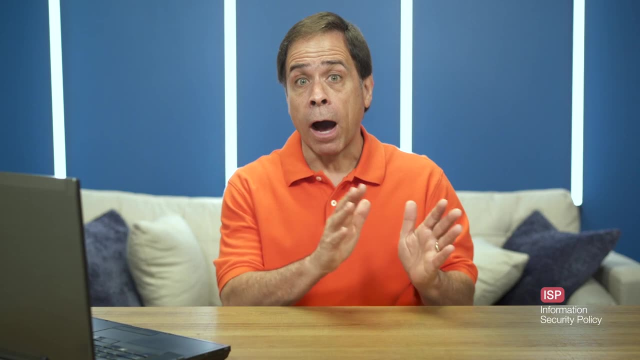 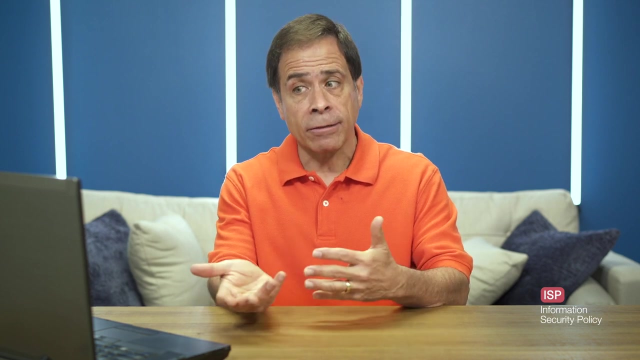 Consider the purpose of a fence around a piece of property. That fence may be there to keep out stray dogs, or it may be there to prevent unauthorized individuals from entering a building. A fence is all about controlling access. Access control is the rules that administer. 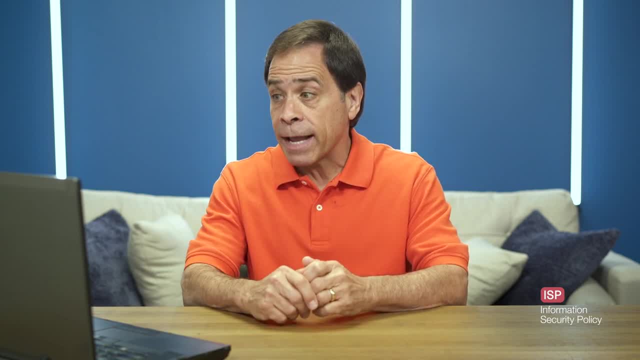 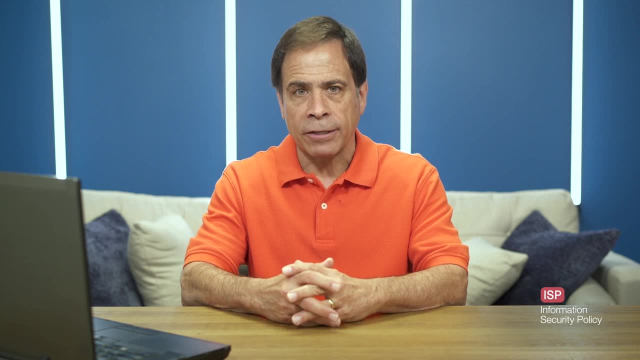 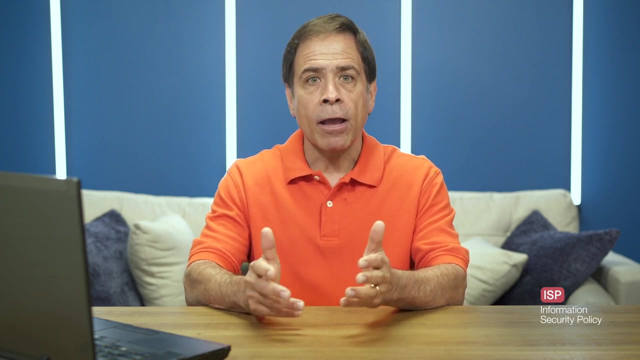 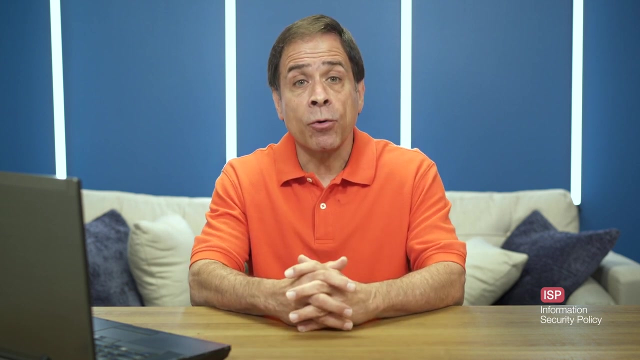 availability to digital assets by granting or denying access to those assets. So an access control policy, sometimes abbreviated ACP, are the high-level requirements that specify why access is managed and who, under what circumstances, can have permission to see those digital assets. Think of files, think of folders, think. 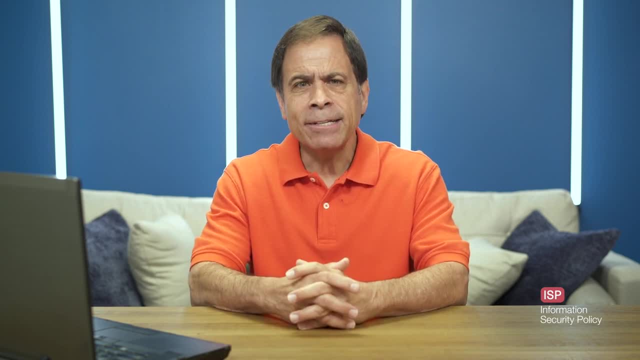 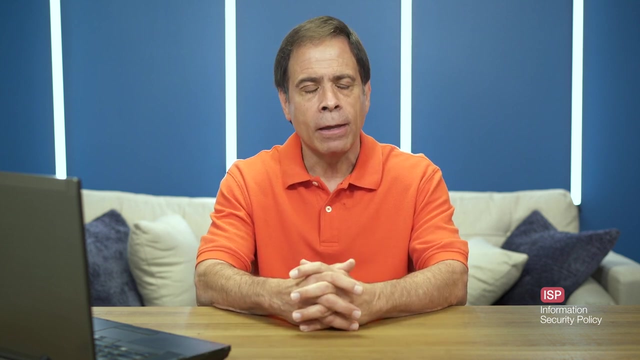 of things on a computer. An ACP access control policy typically has five different areas. The first is the ability to identify the objective of the policy itself. What is this policy all about? Why are we talking about this in our policy? The second area in an access control 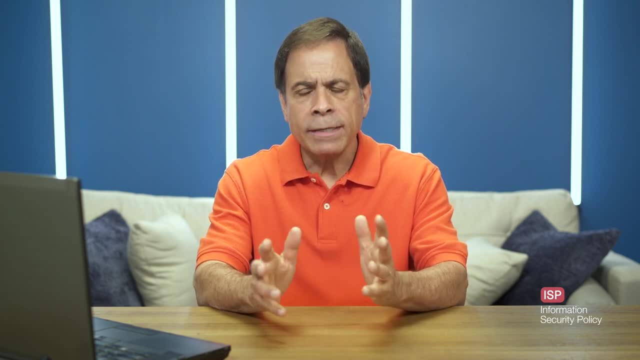 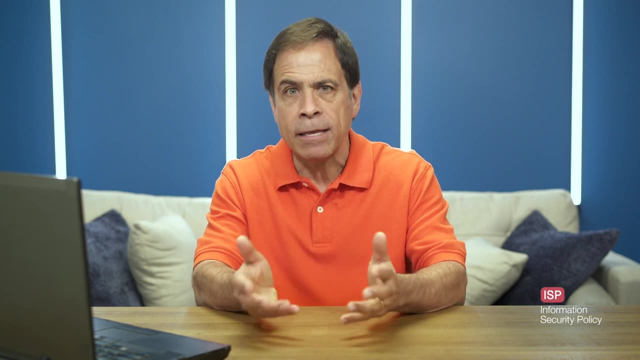 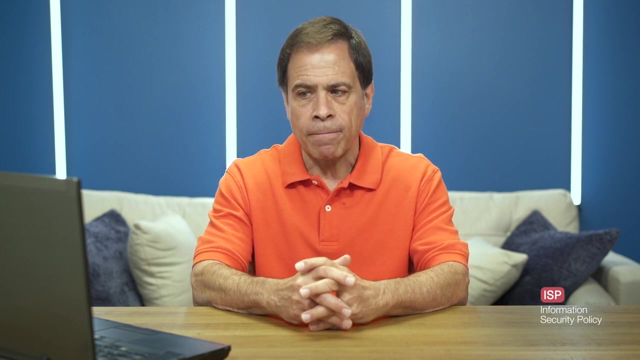 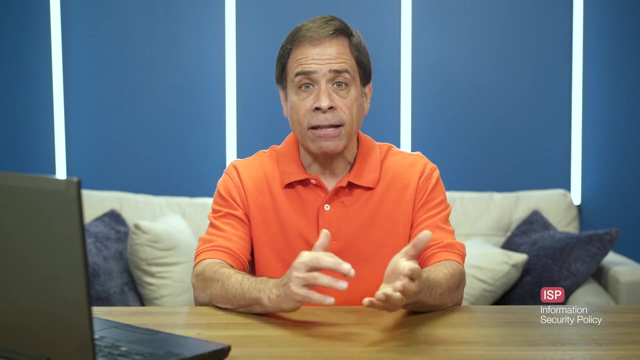 policy. It usually looks at what type of data needs to be protected. Is it HR data? Is it customer information? Is it HIPAA medical data? The third element of an access control policy looks at recognizing a process for identifying individuals to have access to those resources. 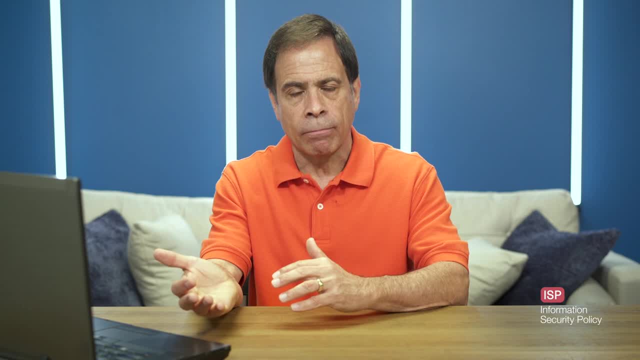 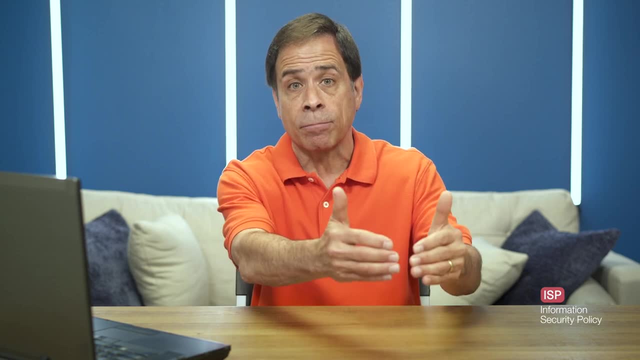 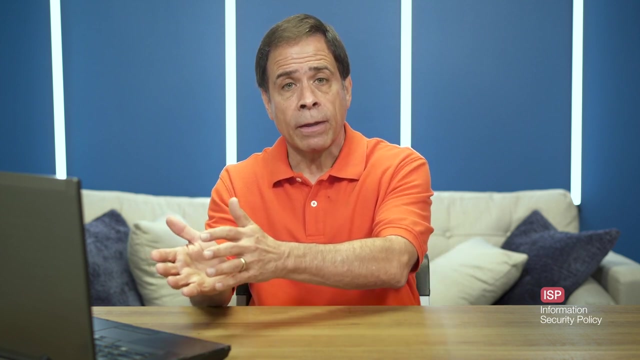 and how exceptions can be granted. In a hospital setting, it might be prohibited that this group of individuals have access to patient data, Yet an exception can be granted by an administrator under these circumstances. That's the why and would be laid out in the policy.